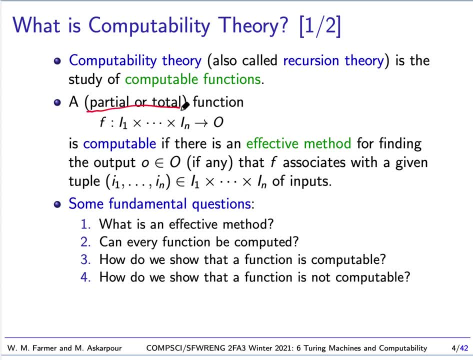 n inputs, and it can be partial or total. say that this function is computable if there's an effective method for finding the output that the function associates with an input or with a set of inputs. So that's what a computable function is. So there's some questions. we 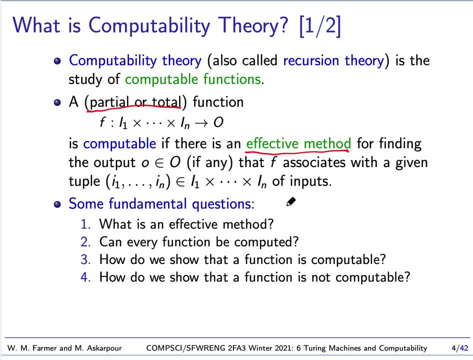 would obviously like to answer: What is an effective method And can every function be computed? We'll find out that every function cannot be computed, and this is why computability theory is interesting and very important. And the third question is: how do we show that a function 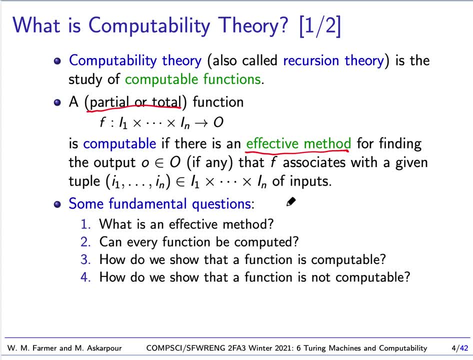 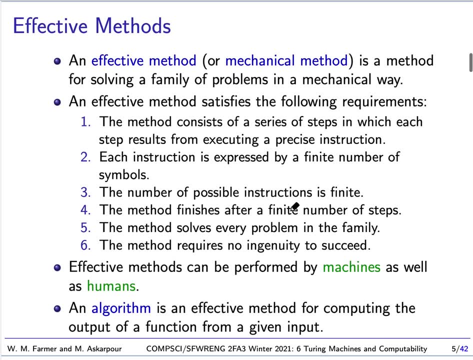 is computable, and how do we show that a function is not computable? So let's start off with an important notion: an effective method. So an effective method which we can also call a mechanical method- Sometimes they're called mechanical methods, Sometimes they're called 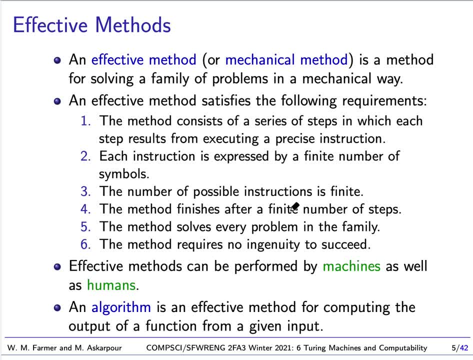 effective procedures. it is a method for solving a family of problems in a mechanical way. So a mechanical way means we can solve it like a machine would solve a problem. An effective method satisfies the following requirements: The method consists of a series of steps in which each step 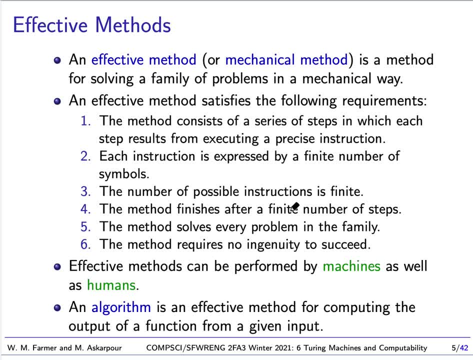 results from executing a precise instruction. So we have a set of instructions and we can execute these one at a time, step by step, and each instruction is expressed by a finite number of symbols. We don't have, in other words, instructions that can be infinitely long. The number of possible. 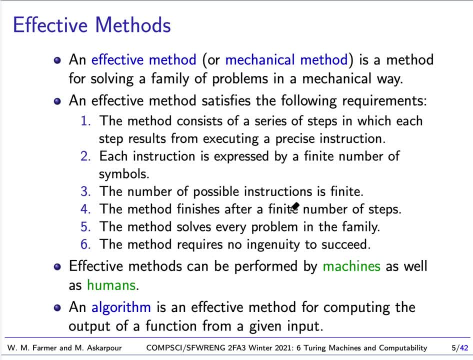 instructions is finite. The method finishes after a finite number of steps and the method solves every problem in the family and the method requires no ingenuity to succeed. Because it requires no ingenuity, the method is not successful. The method requires no ingenuity. 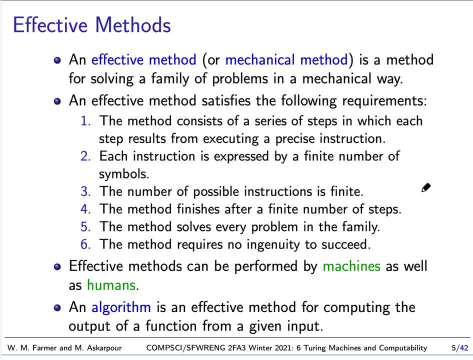 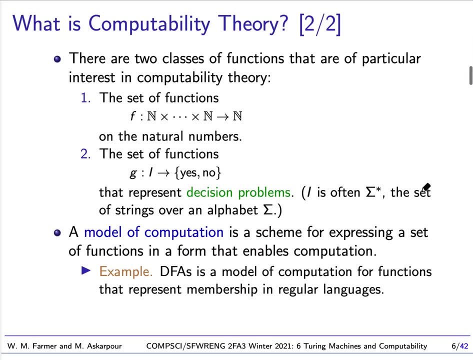 it can be performed by a machine as well as a human, And you're familiar with the idea of an algorithm. An algorithm is just an effective method for computing the output of a function from a given input. Now in computability theory in general, we're considering which functions are. 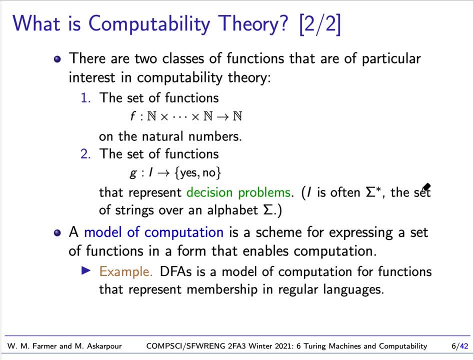 computable, but often our interest is focused on two sets of functions. The first set is a function which is always driven by the packed Eating Curve And very often we think vectorization function, like this function f that takes a certain number of inputs that are natural numbers and 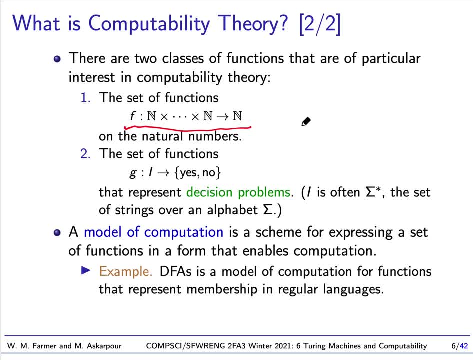 gives back a natural number. so, in other words, the first set are functions on the natural numbers. the second set is a are functions that take some input and give back yes or no. these kind of functions represent decision problems. a decision problem is a problem. where does something belong? 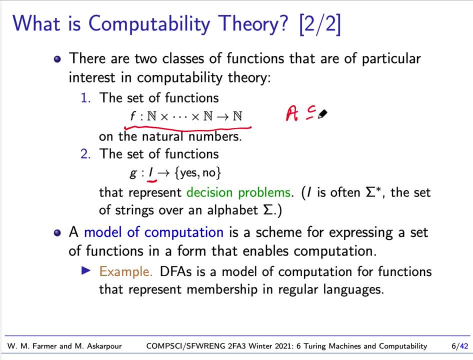 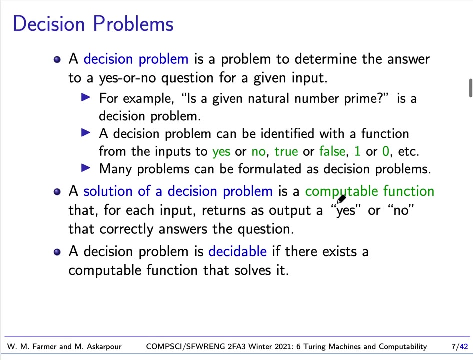 does something belong to a subset of i in this case? if so, we get yes, if not, we get no. and often i is is a set of strings over some alphabet. so let me remind you that about what is a decision problem. a decision problem is a problem to determine the answer. 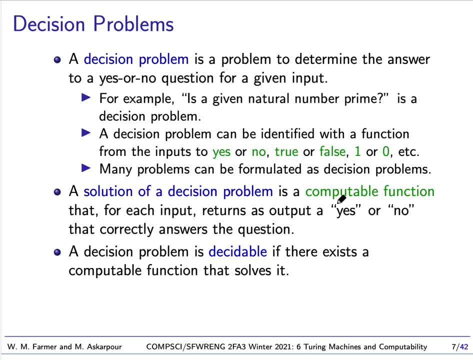 to a yes or no question for a given input. so, for instance, is a given natural number prime? this is a decision problem for a given input. for a particular natural number, we would like to decide whether that natural number is prime or not. now a decision problem can be identified with a function. it's a function that takes 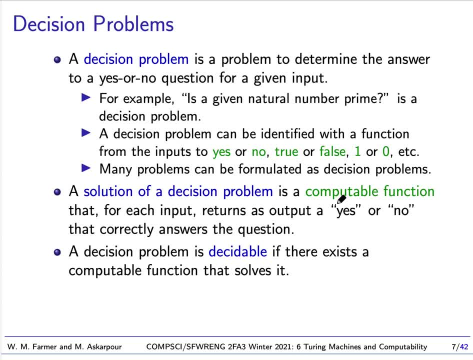 a and inputs and it returns either yes or no, or true or false, or one or zero- any kind of binary answer- and many, many problems can be formulated as decision problems. now, a solution of a decision problem is simply a computable function that for each input returns an output- yes or no. that 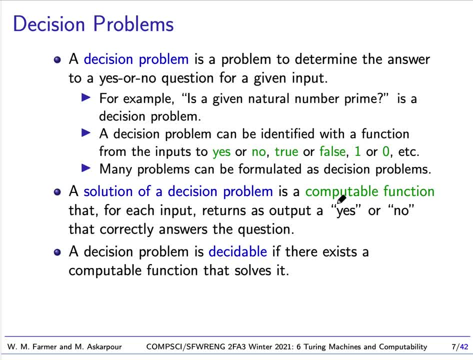 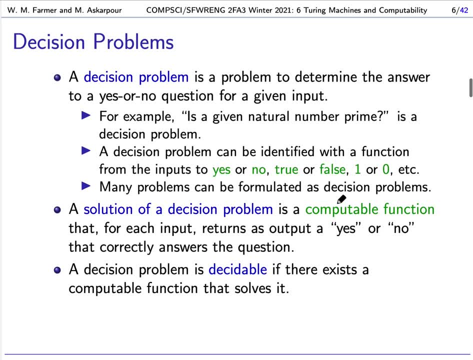 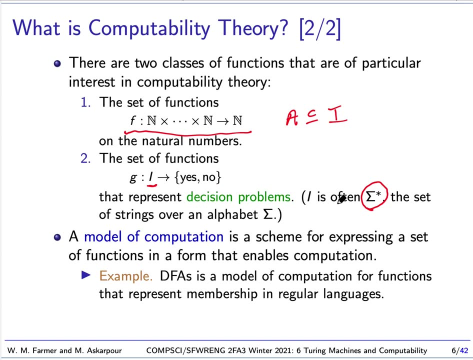 correctly answers the question and this a decision problem- is decidable if there is a computable function and that is a function that solves it. so let me go back up to here. so a model computation is a scheme for expressing a set of functions in a form that enables computation. so it's a way of showing that our functions are computable. 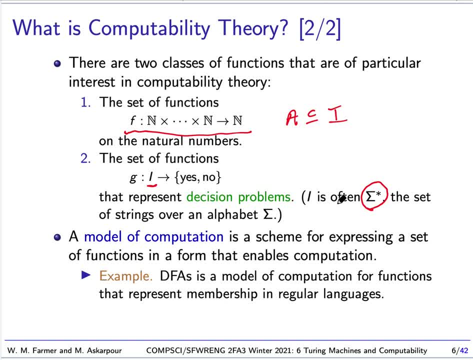 because they're expressed in a way that we can compute with them. so dfa's is a model of computation, of computation for functions that represent membership in regular languages. So if we have a regular language R, we can come up with a DFAA and we can take a string. 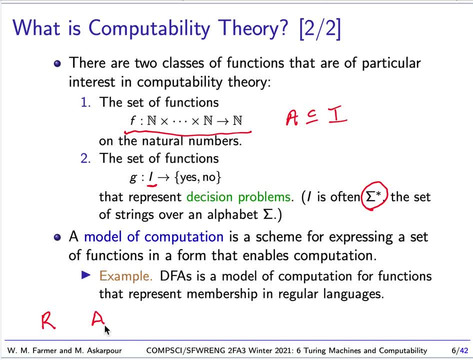 from R and using that DFAA we can compute whether that string belongs. or I should say we can take an arbitrary string. maybe it would be clear if I wrote this: we can take a string which is in some set of strings and we can give it to our DFAA. we can compute. 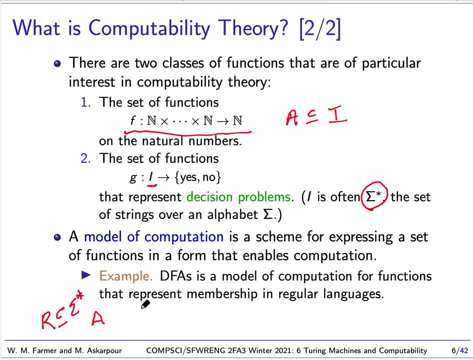 with it and we can determine whether that string is in R or not. So we can ask this question. And so DFAAs are a model of computation for membership in regular languages. We can compute. We can compute whether a string is in a particular regular language by representing that regular. 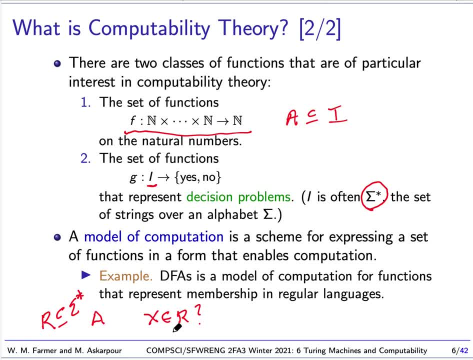 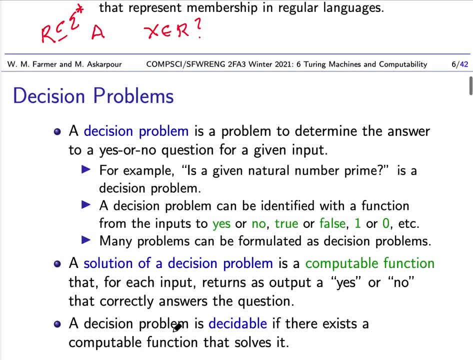 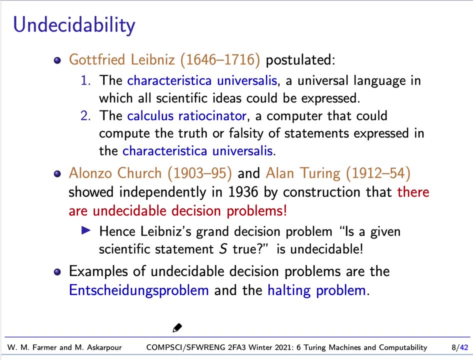 language, using a DFAA, which represents a function that makes the decision Okay. so that's one example of a model of computation. Now the interesting notion is the notion of undecidability, of decision problems that are undecidable. 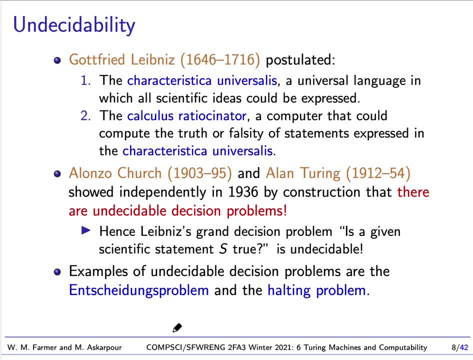 How is a problem undecidable? As you can probably guess, there are no problems undecidable, but there are also no possible problems that are undecidable. How is a problem undecidable? Well, first of all, there is an undecidable function and that's an undecidable function. 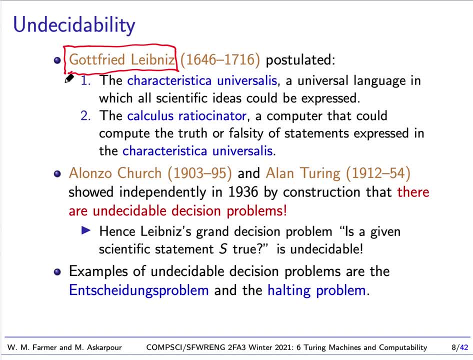 What is an undecidable function? Well, the thing is only one of the main problems that would be undecidable for a person is what is called an undecidable function. It's a simple one, one of the inventors of calculus, But Leibniz did much more than that. Leibniz is one of the most 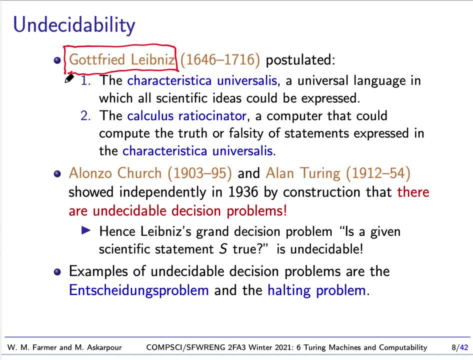 amazing polymaths that the world has ever seen. There's really no one to compare to him that I can think of, except maybe Leonardo da Vinci. He was interested in many things and knew a great deal, And he's probably most famous as a philosopher, but he was trained as a lawyer. 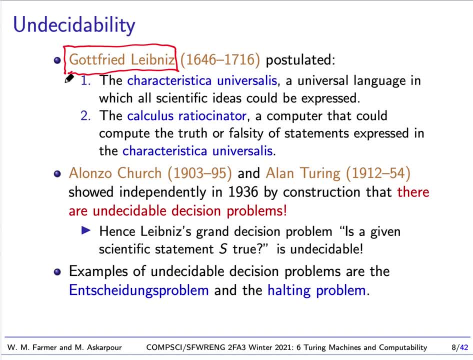 Now, Leibniz was very interested in computing, was interested in computation. He made, or he designed a calculator, a mechanical calculator called the Stoffelwalze, And this calculator was able to do addition, subtraction, multiplication, division and 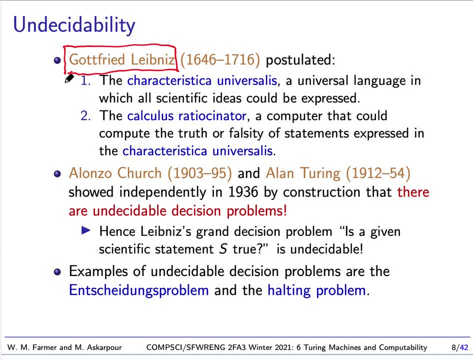 multiplication, And he was able to do addition, subtraction, multiplication, division and multiplication, And he was able to do addition, subtraction, multiplication, division and take square roots. No one had ever been able to create such a machine before, So this is. 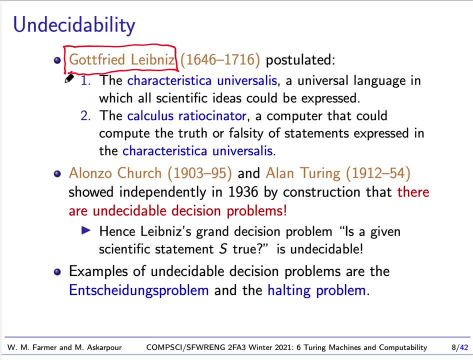 something Leibniz designed and he had technicians built, So he was one of the great, first great computer engineers. Now, Leibniz was fascinated with computation and he really entertained the idea that we can solve problems, many problems, with computation We can. 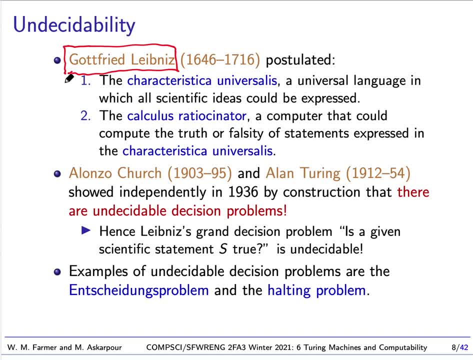 compute answers to our problems, And so he entertained the idea of: maybe we can compute answers to any question. So he developed a language which is called the Characteristica Universalis. Leibniz did all his work, wrote all his papers in Latin, So this is a universal. 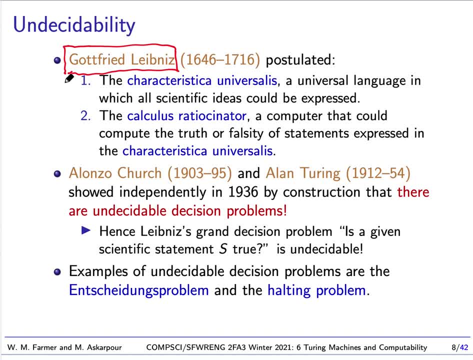 language that he was working on. he was thinking about in which you could express any scientific statement, And in parallel with this, he was also thinking about a computer, which he called the Calculus Ratio Symmetra. So this was a calculator that could take a statement. 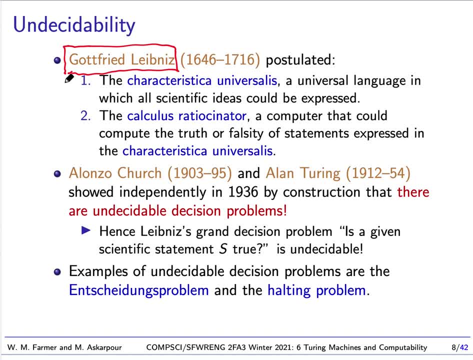 expressed in the Characteristica Universalis and compute the truth or falsity of it. So this is what he's imagining. He's imagining a universal language and a computer that goes with it, that can take any statement written in that language and determine whether it's. 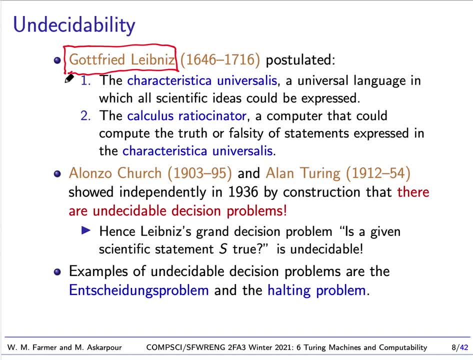 true or false. So this is like the ultimate application of computing to be able to answer any question. And he's imagining reducing philosophy to just writing things down in the language and plugging them into the calculus rationator and getting out an answer. 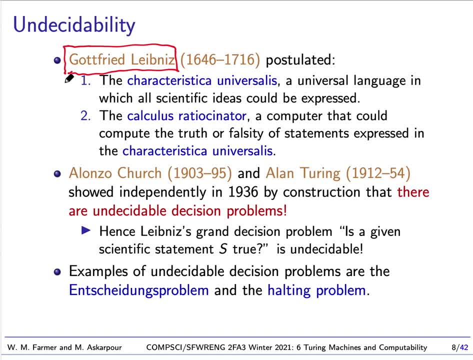 Now the interesting thing is: is this all an impossibility? Was there any hope that this could actually happen? Well, no one really had an answer for Leibniz for about 200 years, until two logicians, Alonzo Church and Alan Turing, both independently in 1936, they show that there are undecidable. 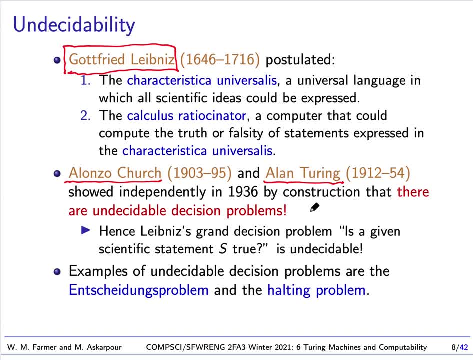 decision problems. They show that there are decision problems for which we cannot compute the answers, And they did this by construction, which means they actually produced. they described the actual decision problems that could not be decided, And so this shows that Leibniz's grand decision problem is a given scientific statement. true. 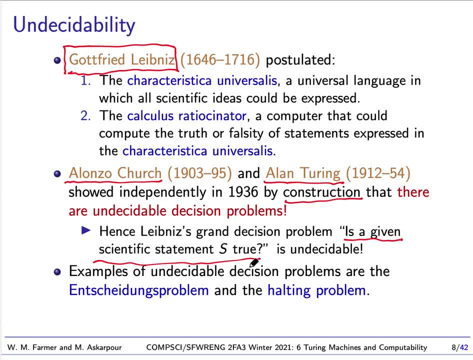 this is an undecidable problem And, as a result, it took 200 years to show that Leibniz's dream is not possible. Now, examples of undecidable decision problems are the. the two, probably two. first examples are the Entscheidungsproblem. 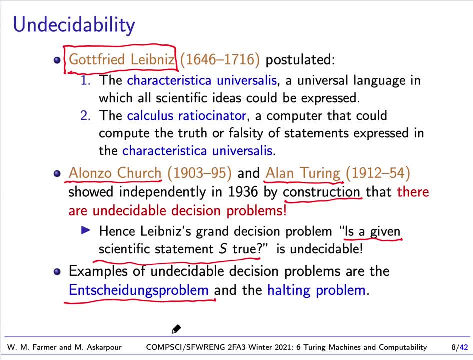 This is a problem of whether, of determining whether a statement you write in first-order logic or some other logic is valid or not, And this is the problem that Church showed was undecidable. And another problem is a halting problem. If you have a programming language, you would like to know whether a given program halts. 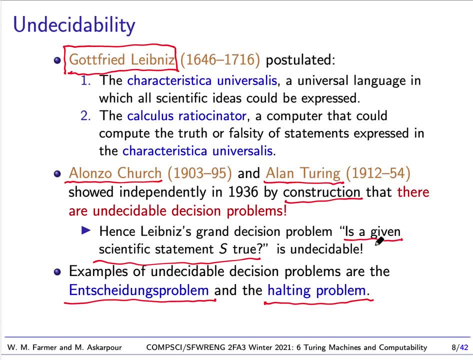 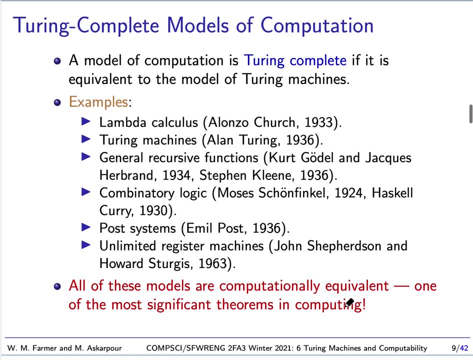 or not on a given input. So Alan Turing showed that this was not the halting problem, was not decidable for a particular model of computation. Okay, so there are many kinds of models of computation, but there's a special class of these models. 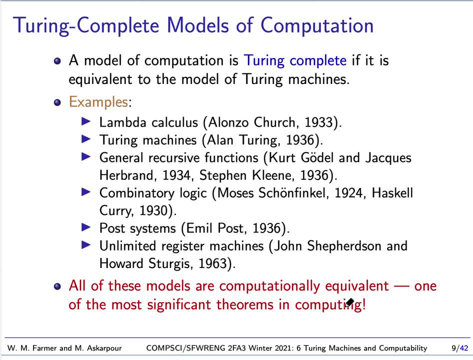 Which we now call Turing-complete models. So one of the models of computation is the model of using Turing machines, which we're going to look at in much more detail as we go through this topic. So a model is Turing-complete if it's equivalent to the model of Turing machines. 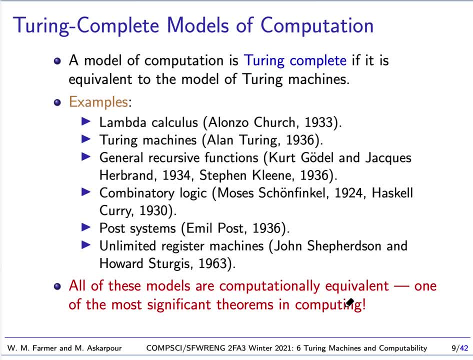 And in the 1930s a bunch of- well a group- of these models were developed. So Turing developed a model called the Lambda Calculus in 1933, and people are still very much interested in Lambda Calculus- Turing in 1936 developed a model called based on Turing, what we now call Turing machines. 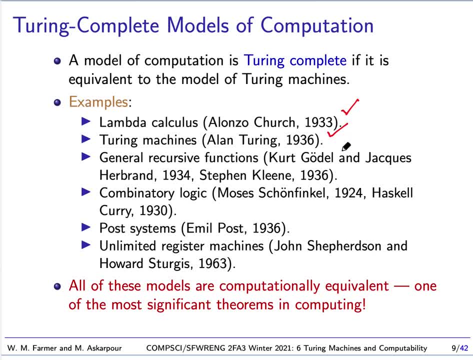 which are abstract, idealized machines, And another model is general recursive functions which people are very interested in today. This was developed by Kirk Gehl and Jacques Ebran in 1934, but it was very much developed by Stephen Kleeney a few years later. 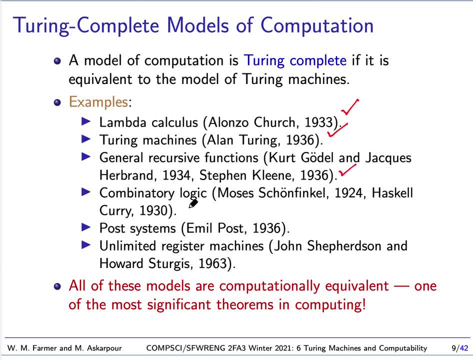 Another model of computation is combinatorial logic, which today is still a model people are very interested in. Combinatorial logic was developed by Moses Schoenfinkel- Okay, But it was really developed a great deal after that by Haskell-Kreuth. 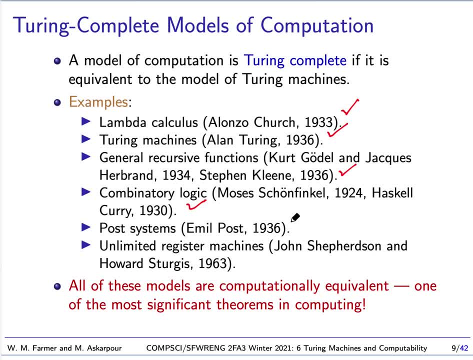 And the last model I'm going to mention in this group of models that come from the 1930s are POST systems. This was developed by Emil POST, So these were early models of computation, which happen to be all equivalent to Turing machines. 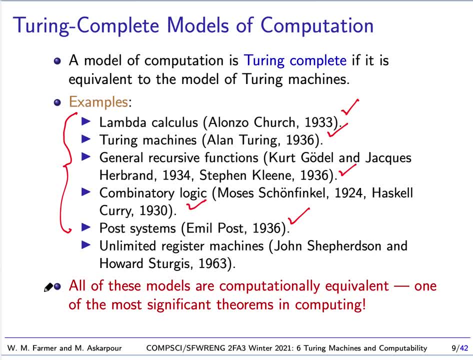 and so they're all equivalent to each other. Now, since the 30s, many other models have been developed, but I want to mention one model in particular, one Turing complete model in particular. This is the model of unlimited register machines developed by John Shepardson and Howard Sturgis. 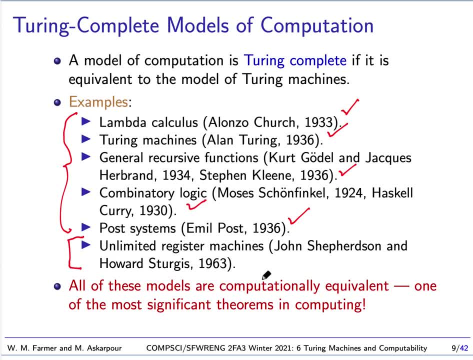 This model is interesting because the machines, these abstract machines, resemble how modern computers look. The machines are based. The machines are based on a bunch of registers and you can move numbers- natural numbers- back and forth between these registers And the machines are unlimited in two ways. 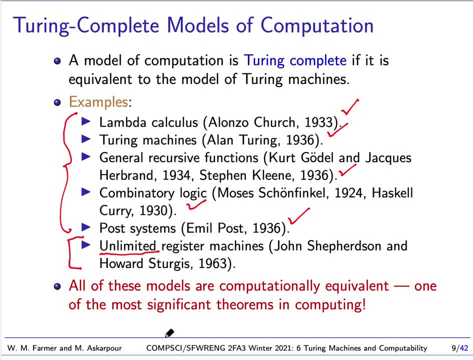 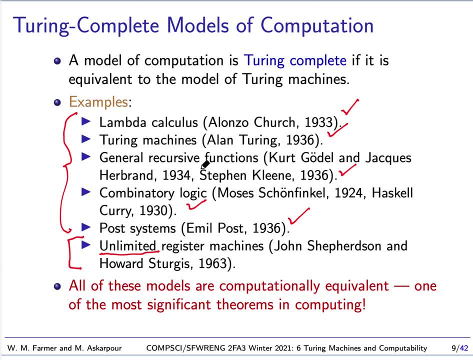 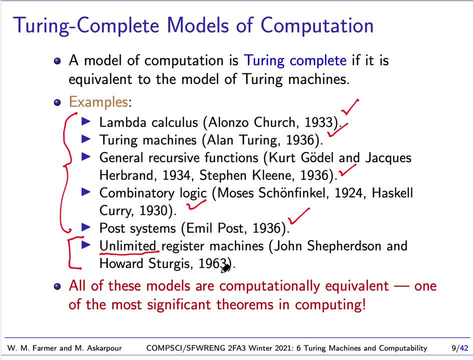 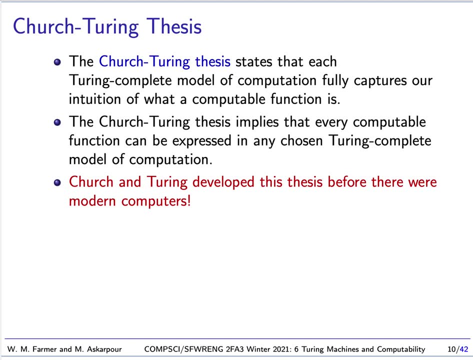 On the surface, there's no reason to believe that they're equivalent, but they are. They're equivalent because there's some basic idea about computing that all these models capture. So Church and Turing. So Church and Turing, they stated a thesis. 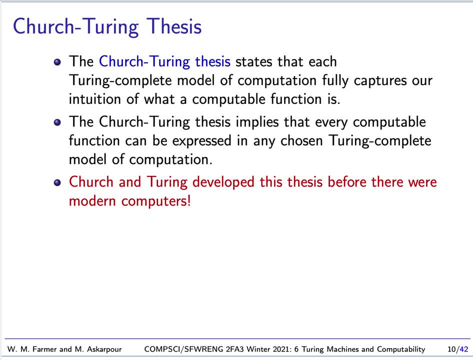 And the thesis says that each Turing complete model of computation fully captures our intuition of what a computable function is. So what this means is is anything that we can express with one of these models is computable, and anything we can't express is not computable. 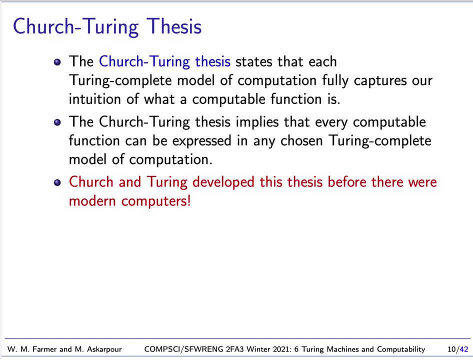 Now there isn't a mathematical proof of this, but no one has ever ever come up with a function that we, that people, would say is obviously computable, which is not representable in one of these Turing complete models of computation. Now one way you can apply the Church-Turing thesis: 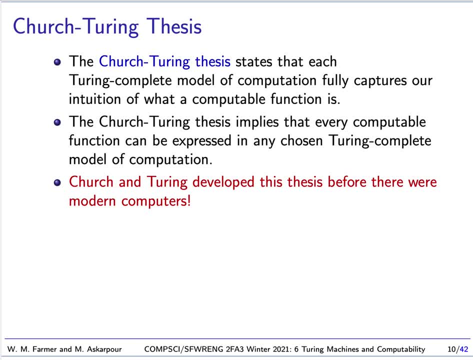 is if you were working on something and you came up with a function that was computable and you asked the question: well, is this computable? According to the Church-Turing thesis, you would if it's, if you think it's computable. 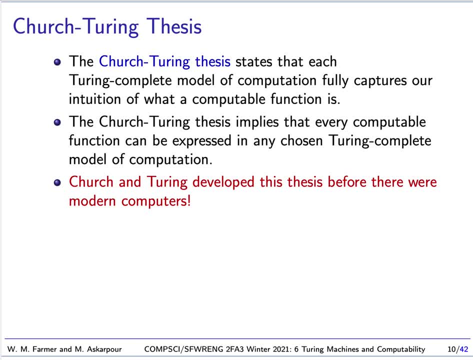 if people agree it's computable, then it will be the case that you can express this function in any of the any Turing complete model of computation that you choose, And so it. so it really seems, according to the Church-Turing thesis. 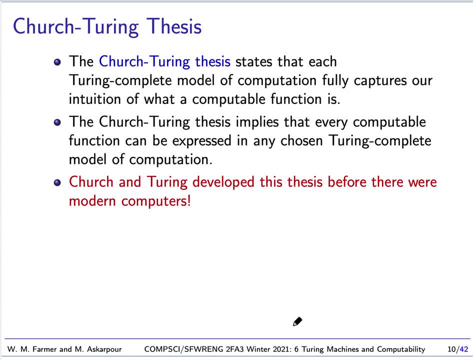 we know what computation is. We know what computable function is. Computable functions are the functions that we can represent in a Turing compute, Turing complete model of computation. So the really interesting thing is Church and Turing developed this thesis before there were modern computers. 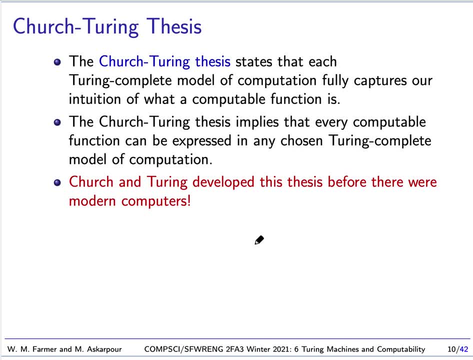 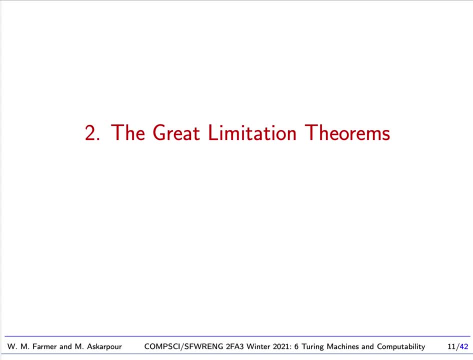 Okay, so we're going to stop here. This will. we'll continue next time with the great limitation theorems. See you then. 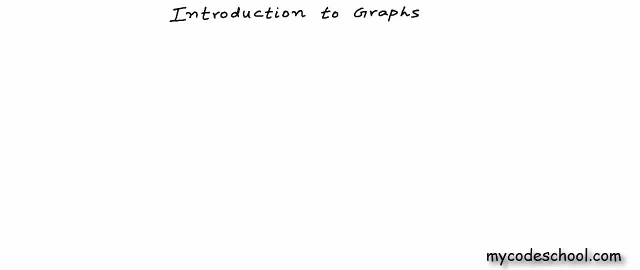 Hello everyone. So far in this series on data structures we have talked about some of the linear data structures like array, linked list, stack and queue. In all these structures, data is arranged in a linear or sequential manner, So we can call them linear data structures. 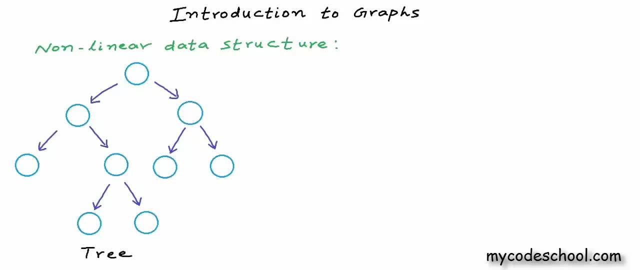 And we have also talked about tree, which is a non-linear data structure. Tree is a hierarchical structure. Now, as we understand, data structures are ways to store and organize data, And for different kinds of data we use different kinds of data structures. In this lesson, 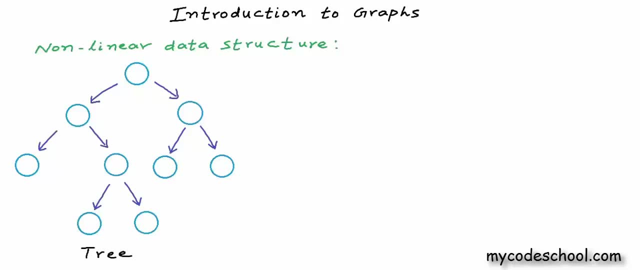 we are going to introduce you to another non-linear data structure that has got its application in a wide number of scenarios in computer science. It is used to model and represent a variety of systems, And this data structure is graph. When we study data structures, we 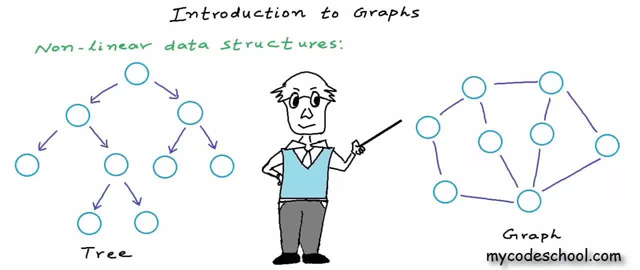 often first study them as mathematical or logical models. Here also, we will first study graph as a mathematical or logical model And we will go into implementation details later. Okay, so let's get started. A graph, just like a tree, is a collection of objects or entities. 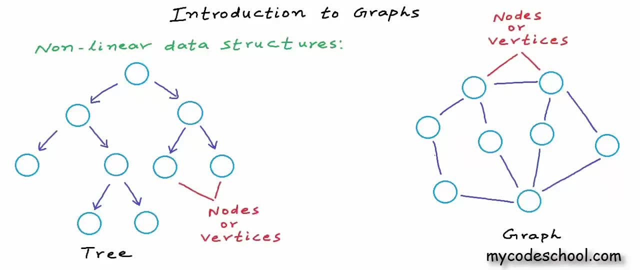